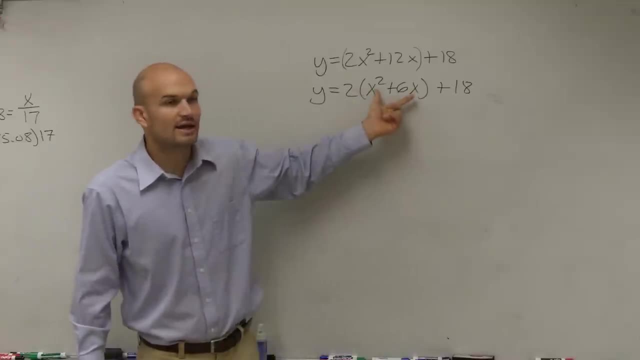 Now that we have a A equals 1. And we have a binomial in here, What we need to do is create a perfect square trinomial. So, to create a perfect square trinomial, Yes, Could we factor the 2 out of 18 also? 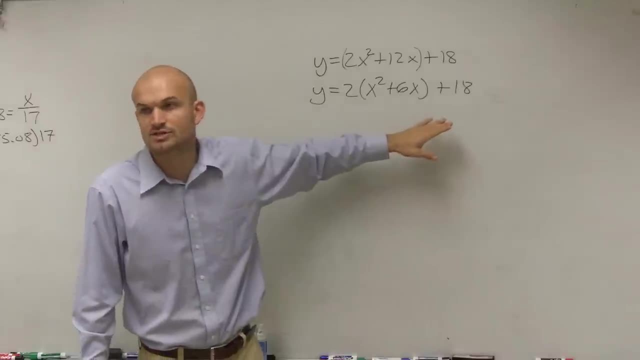 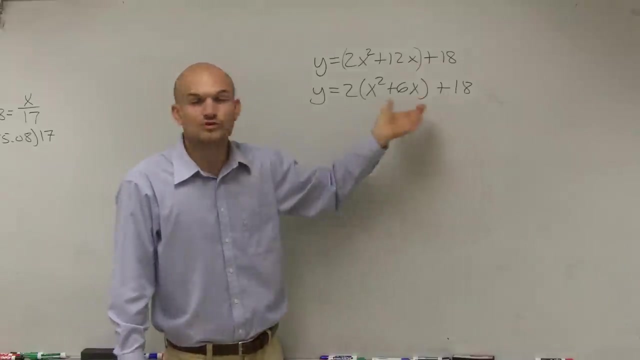 You could, You could. However, I just prefer just to kind of go through it this way, Just because I just like dealing with factoring out of these two terms and not dealing with the 18.. But yes, you can factor out the 2 out of the 18.. 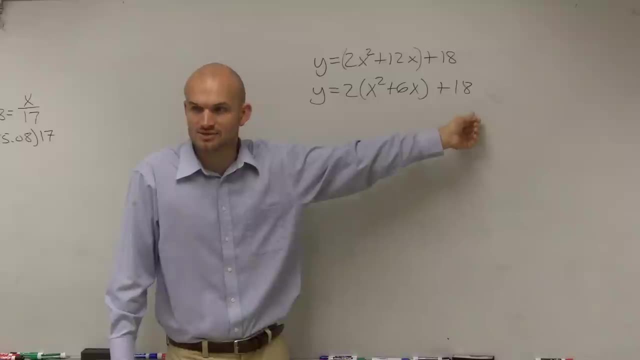 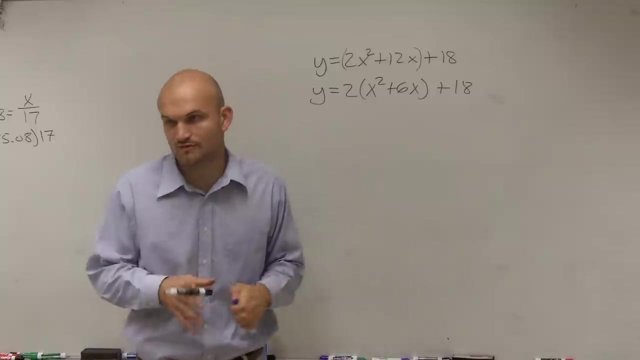 The only reason why I don't like doing it is because then you have to remember just to multiply back Out it again. So I always just like to keep it just without the factored out of the 18.. But yes, you could factor 2 out of that 18.. 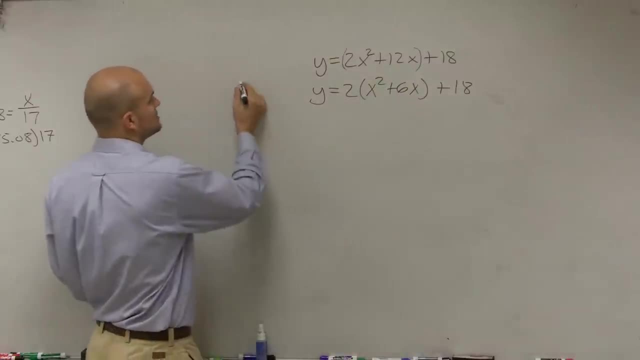 So now what I can do is to determine the perfect square is. I'm going to take Destin, I'm going to take 6 divided by 2 and square it Where 6 is my b. So 6 divided by 2 is 3.. 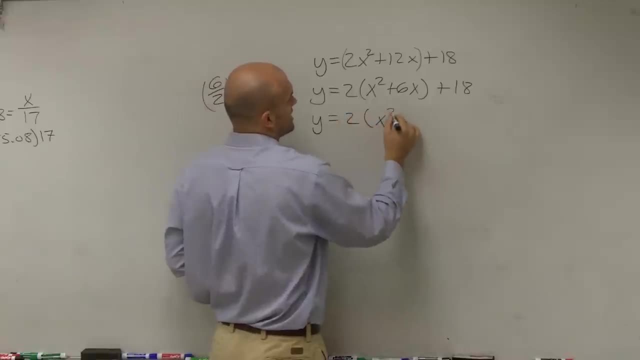 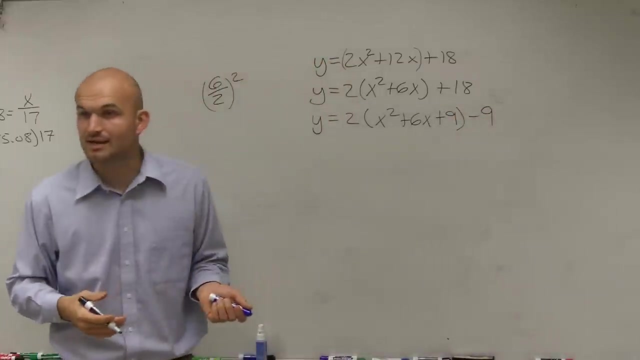 3 squared is 9.. So I write: y equals 2 times x squared plus 6x plus 9.. And then, remember, I also have to make sure I subtract 9 on the same side, But remember, I'm not really adding and subtracting 9.. 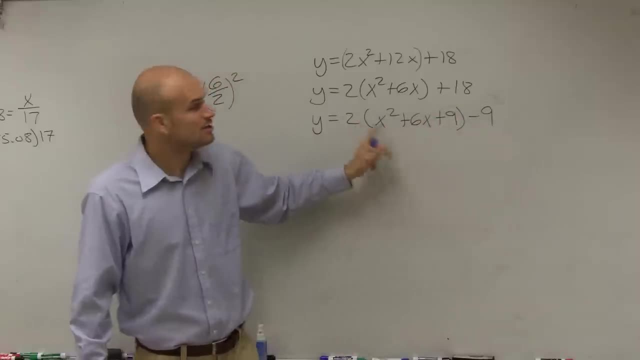 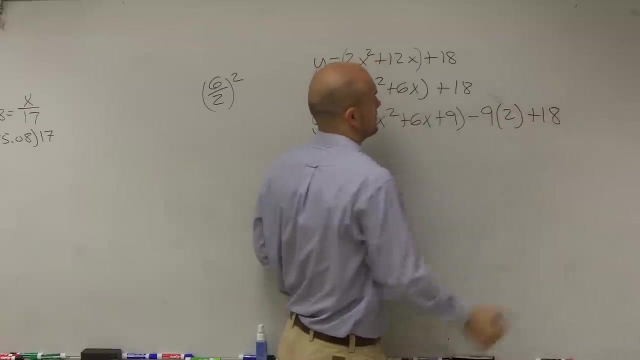 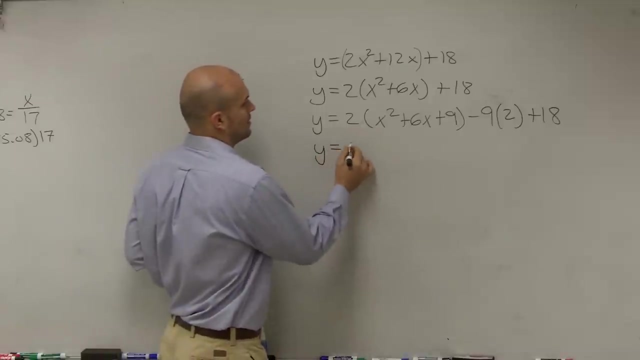 Because I'm adding 9, that's being multiplied by 2.. So I'm going to have to subtract a 9 that's going to be multiplied by 2.. Okay, So now when I go ahead and complete my square, I can say: well, this is the perfect square trinomial. 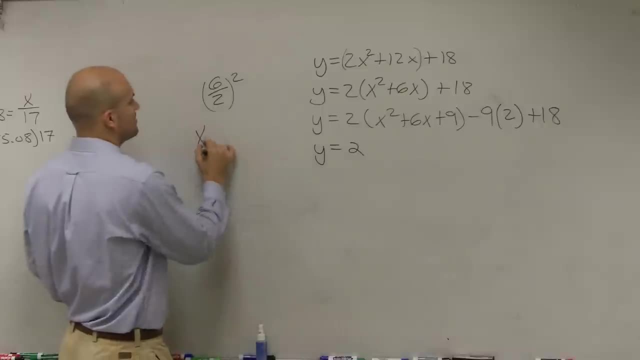 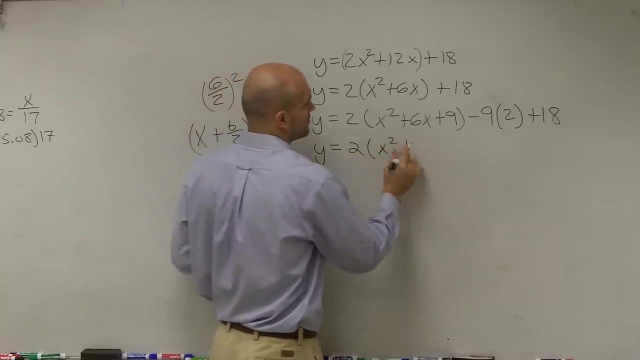 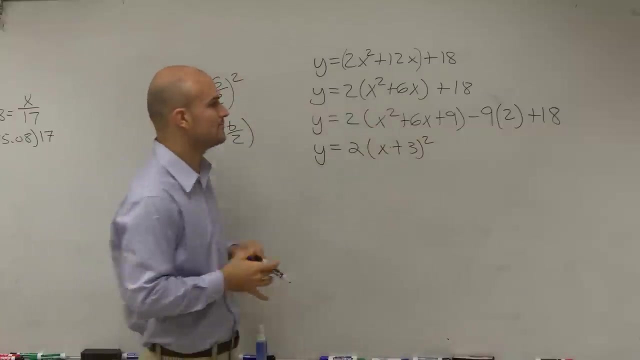 So what does it look like as a perfect square? Well, the one way we can always remember It is x plus b divided by 2.. Well, we said, b divided by 2 is 3., In which we know that x plus 3 squared is the same thing as your perfect square trinomial there. 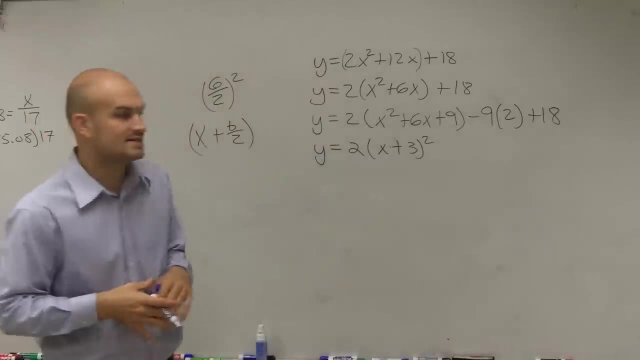 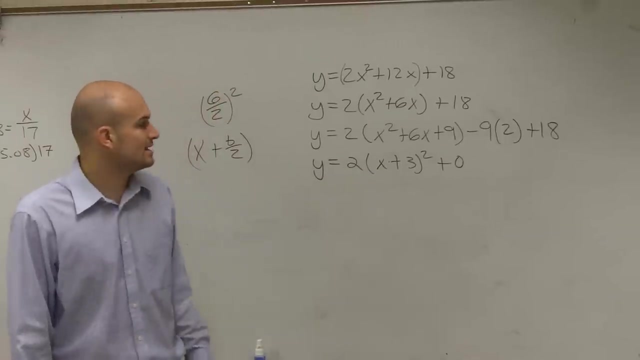 Therefore, negative 9 times 2 is negative, 18 plus 18 is 0. So we can just write in the 0 just forward, so we can use it in vertex form. So now you guys can see that here is our same exact problem, but now it's in vertex form. 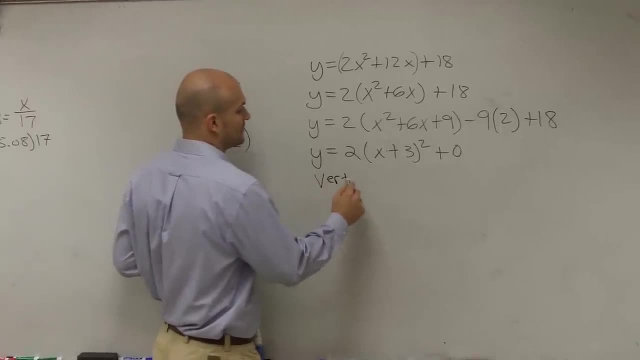 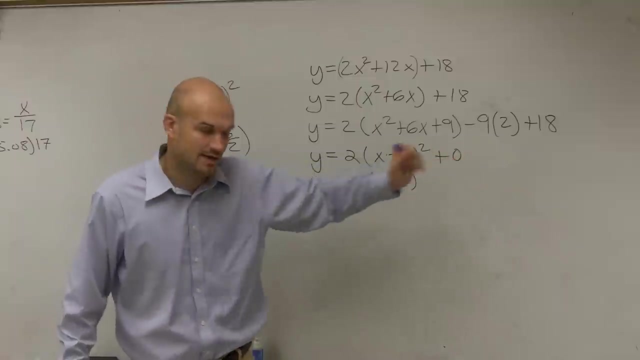 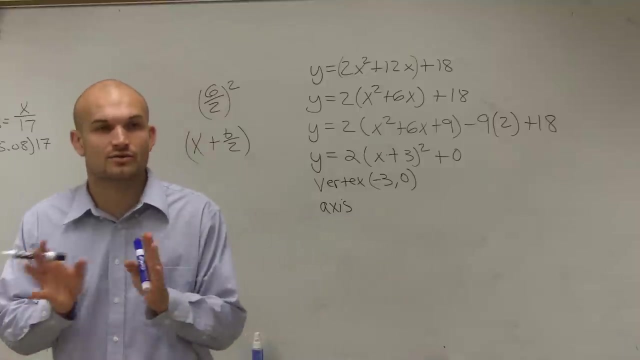 Well, since it's in vertex form, our vertex is going to be negative: 3 comma 0,, right Where your vertex is your h comma k. Then we have our axis of symmetry, And remember, the axis of symmetry is going to be the vertical line that your parabola is going.